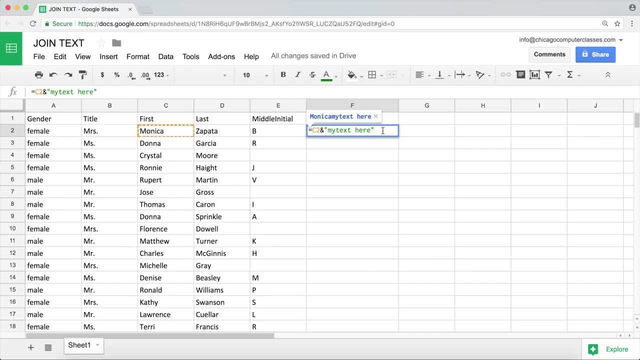 multiple numbers together. you can do this plus this, plus this, And in this case we're saying: let's take the C2, then this plus sign for text, which is our ampersand plus our text, And then we can do another one of those signs which is adding again, And then we can add something else like this one: 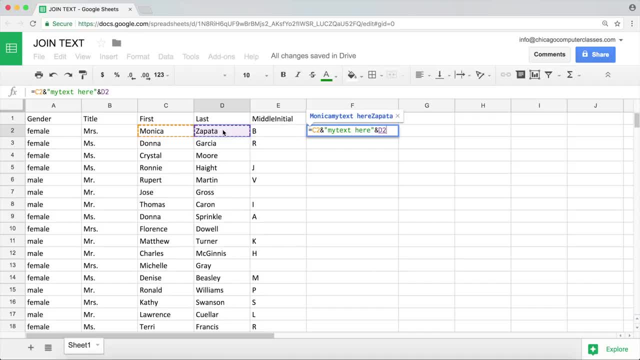 So now it should be the first name, whatever text I provide, and last name. So if I hit enter, that's what I get Now. finally, if I get back now, I'm going to replace this text that I have with a space. 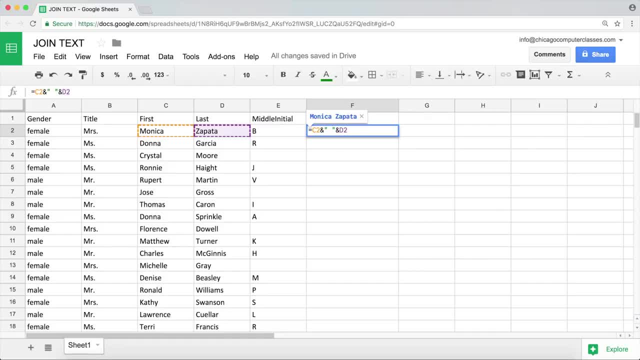 That I want, which is going to be simply a space. So if I had enter, that's our first and last names And if I copy this down, that should be our first and last names. So that's a way to get our first and last names. 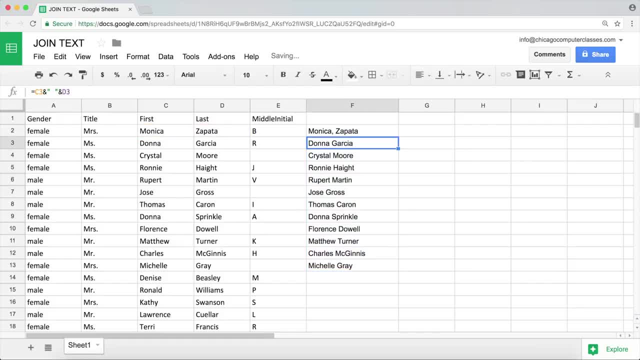 Now, obviously you could have done other things other than a space. If we wanted, like a comma space, you would do comma space. copy down: you have first and last names separated by a comma, right? So that's one way to do this, which is the and sign. 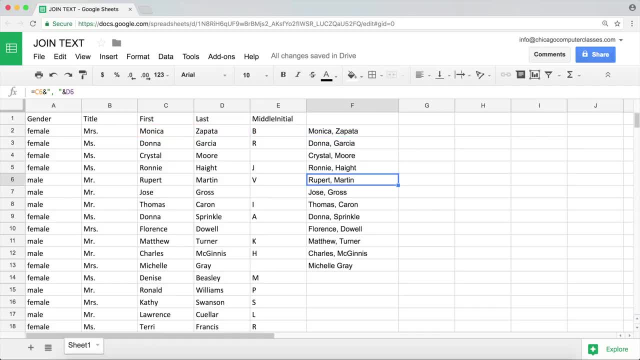 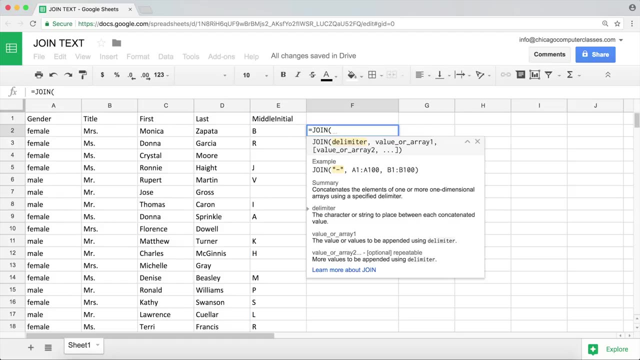 To join text together. Now let's try to use a different method When I go back. another way to do this is to use a function called join in Google Sheets, And the first thing is the delimiter. So delimiter is what it is that I want to. 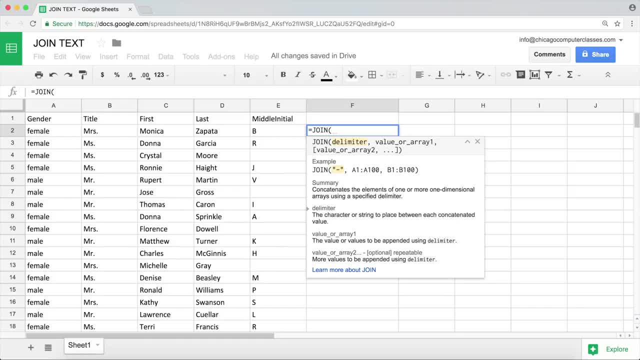 use in the middle of different pieces of text that I combined. So, if you remember, what I did was the space. Now what I'm doing to do is that delimiter. So I'm going to do code space quote, because it's text comma, and the next one is the values that I want to merge. So you have a couple of 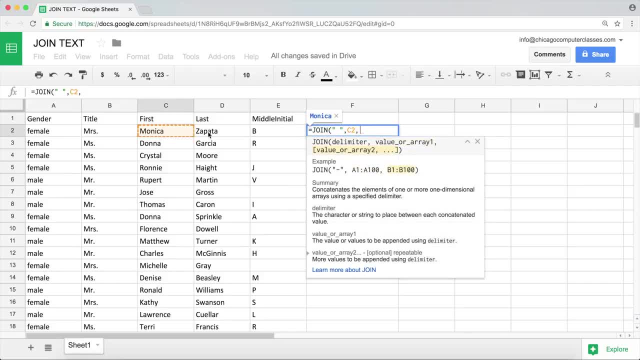 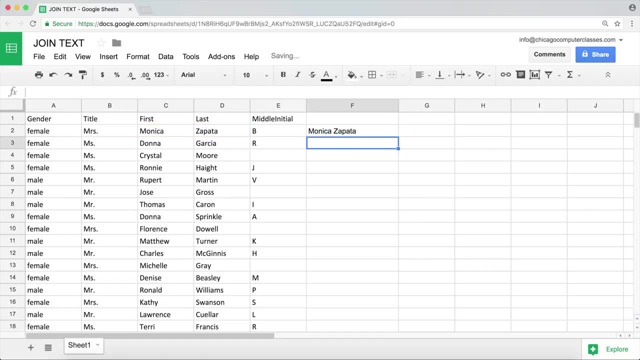 options here. you can either do this comma, this, So I'm basically comma separating the first one and the second one I want to add, And if I hit enter I'm going to get that. But I can also simply just provide a range which is this And I: 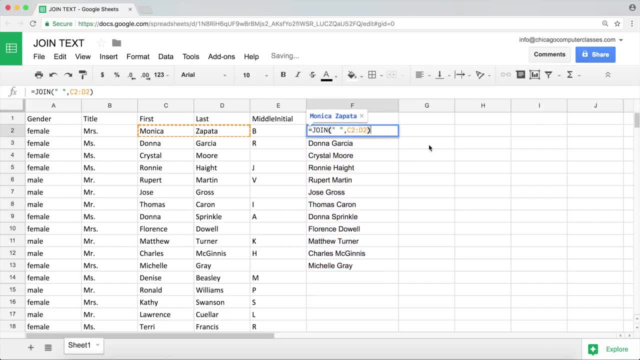 would get that result: First and last names. So that's our join formula And obviously the same way you could have done a different separator and get results like this. So that's first and last names combined. Now let's say, not only we want to combine first and last names, we 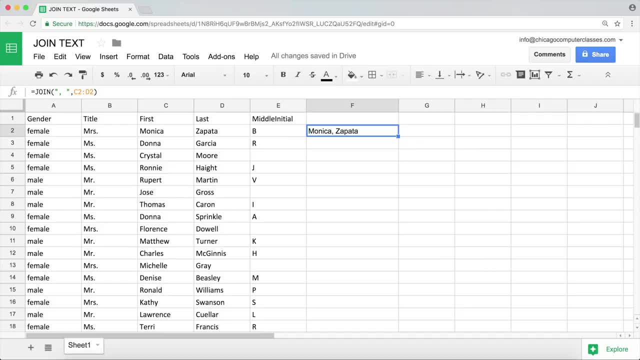 also want to possibly do the middle initial and maybe even the title. So we want the full name for everybody here. So what I'm going to do, I'm going to go and start by join, And what I want as a separator is my space. So what I want, I want it. 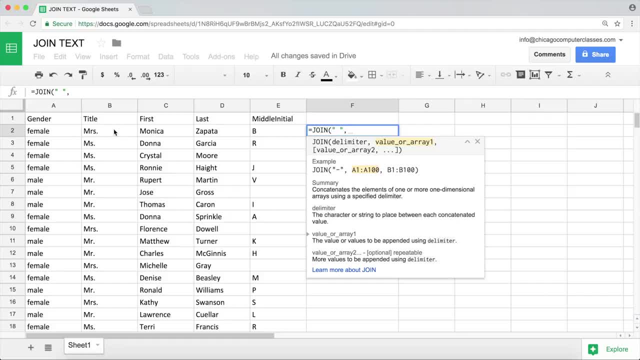 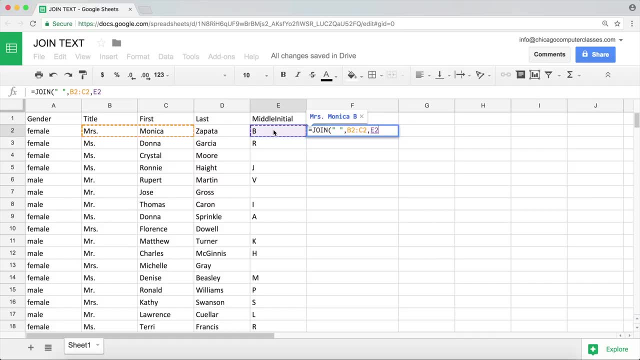 to be the title And then the first name. I'm going to do come on at range, And then I want the middle initial comma here and then last name, And then I'm going to do come out And there it is. That's our separators. So that's pretty good, But if you pay attention, right. 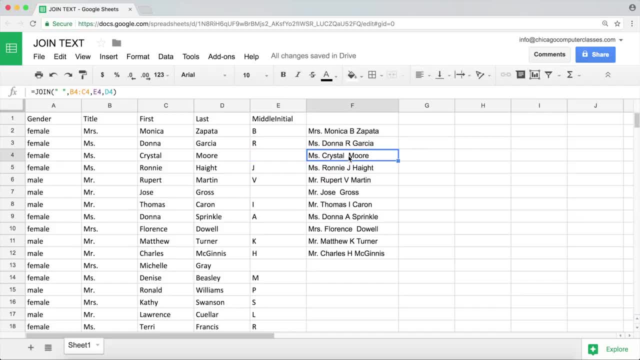 here. if we have missing middle initials. we're going to get two spaces here Because basically we said that the separators we want is the space right, And it's going to put space between each one of these different cells that we have Now in the. 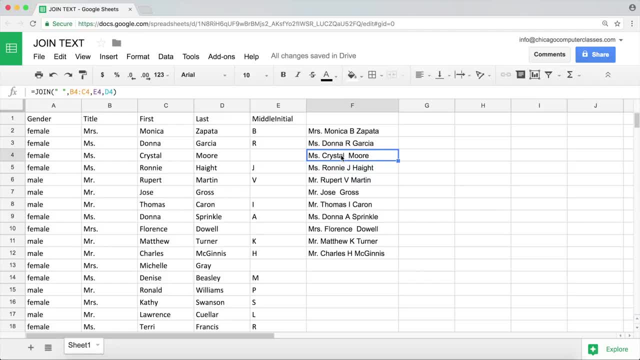 this particular case: after crystal, which is the first name, we then have a space, and then middle is usually nothing, But after that we still put a space. So we have two spaces. there are a couple of ways around this, So one way should be by using 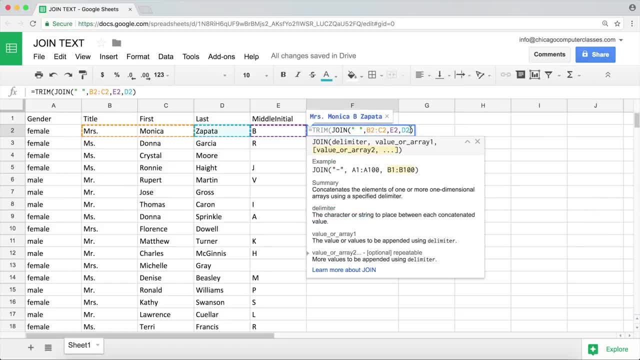 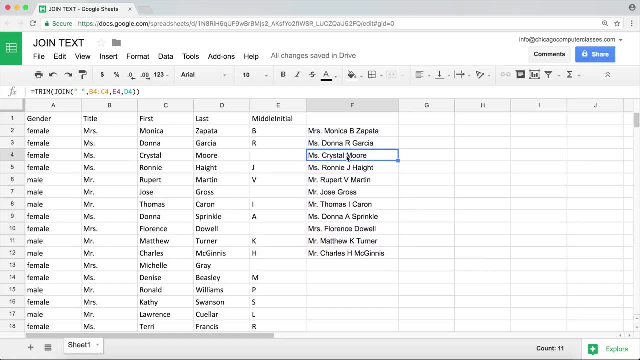 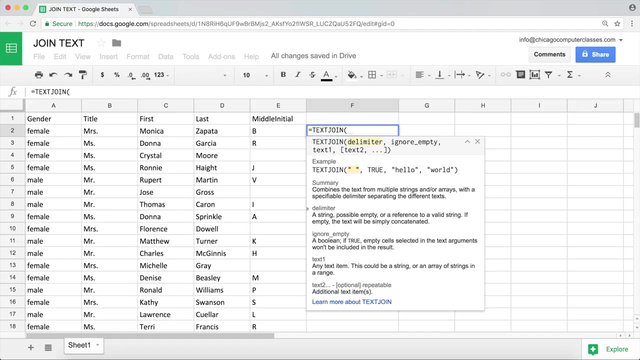 trim function. So I'm going to try this out. And there it is. that's our trim function, and trim removes unnecessary spaces. And now we're fine. That's one way to go around this. So that's trim. Now, another way to do this is by using another function that's called text join, And text join is 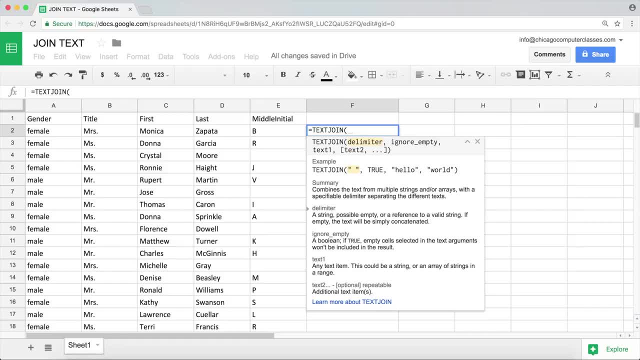 similar to join, but it has an extra option, And that extra option is whether it should ignore empty cells in the range that you provide or not. So right now, the first one is delimiter. So, again, my delimiter is a space comma. then do you want to ignore empty cells or not? So what I'm going to say is true, I do. 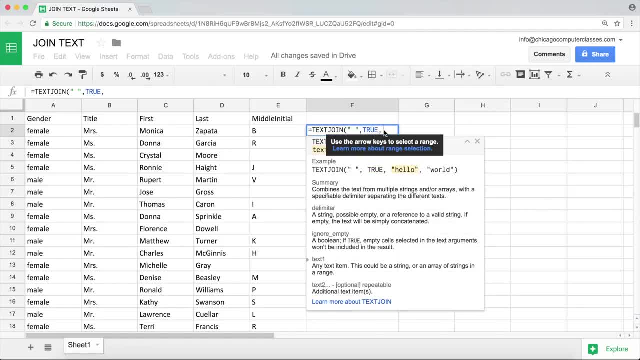 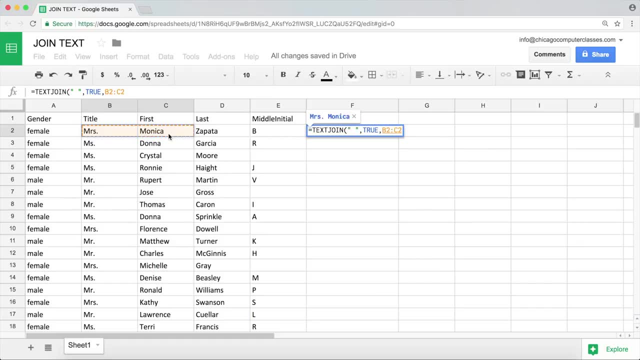 want to ignore empty cells. So true for that. And the rest is kind of the same. So I'm going to do my first one, my title and first name comma, then I'll do my middle initial comma and then I'll do my last. 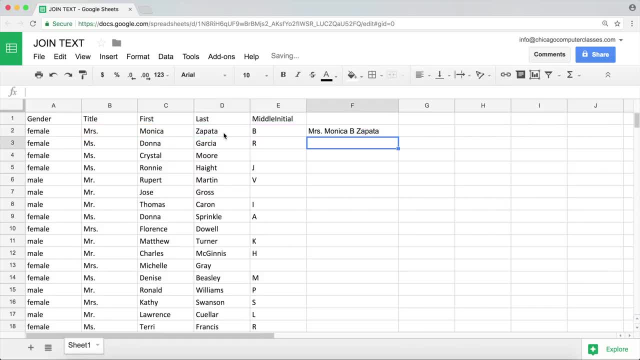 name. Close the parentheses. hit enter. there we have it Roll, push it down and you can see how we have all these missing ones. we're basically just ignoring that extra space. So that's our text join function. So again works similar to join. the only difference is you have this extra. 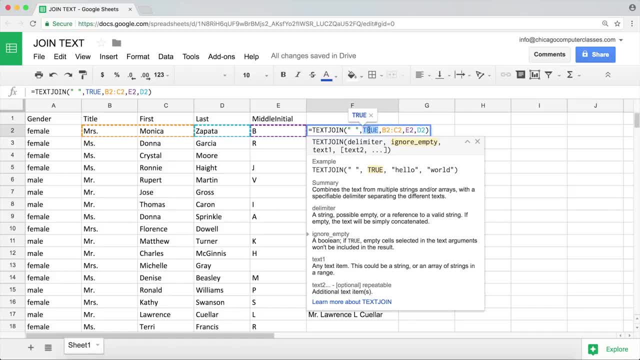 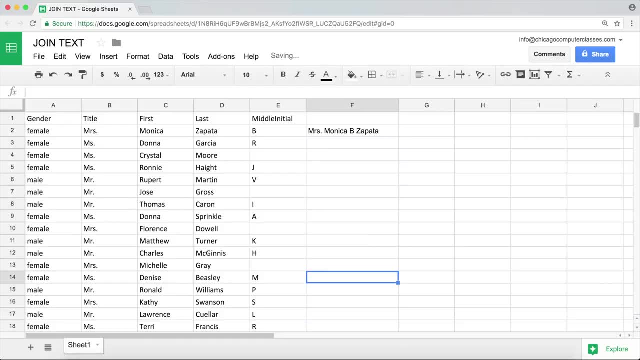 argument here that you can add as true or false. So that's our text. join. Now let's say: what I want as a result is not what I have here, So let me just copy and paste the values only here. What I want is this: So it's going to be the title, the first name, then I want this middle initial. 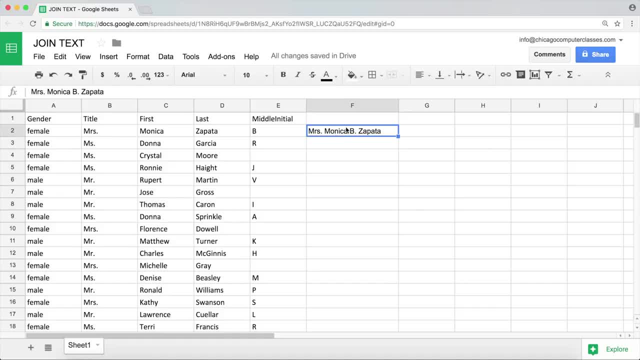 with a period after that and then the last name. Let's try to do that. So I'm going to go here and start with my join function, What I said I wanted. I said I wanted the title, then the first name, right So separated by a space. So there it is. that's the title, and 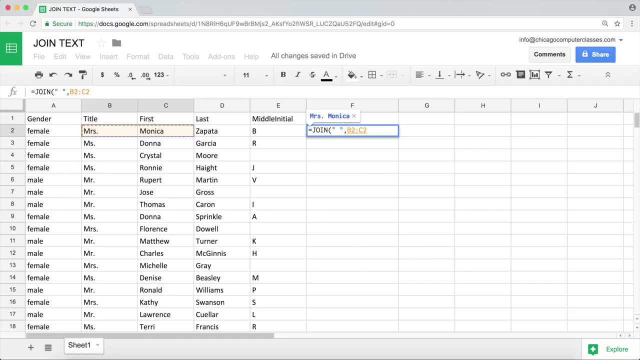 the first name And then after this, I want a space and middle initial right. So I'm going to do this middle initial. so do this, let's see what we get. so we got this. so let's see what we have now in this particular 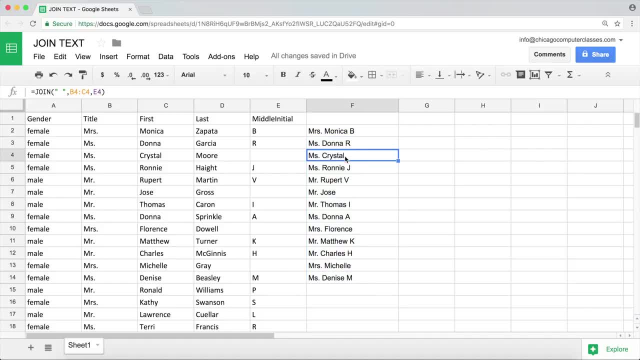 case. we have an extra space here. it's invisible, but it's after crystal. because of the same problem. we have the joint right that will treat those extras the way it treats them now. what we want after that is basically, we want a period after each one of this initials the problem with that. 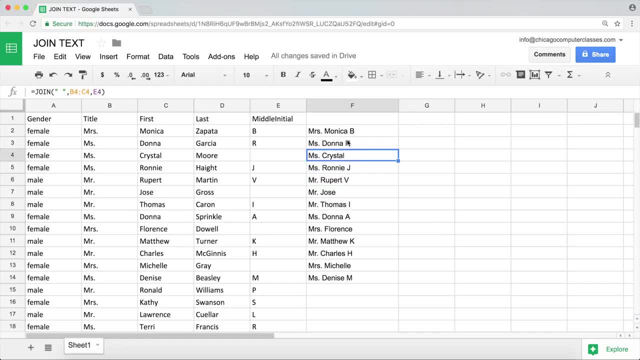 period is that we only want that period when the middle initial exists, not when it doesn't exist. so what I'm going to do, I'm going to adjust this formula and I'm just going to use join to simply just concatenate the title and the first name. so so far. 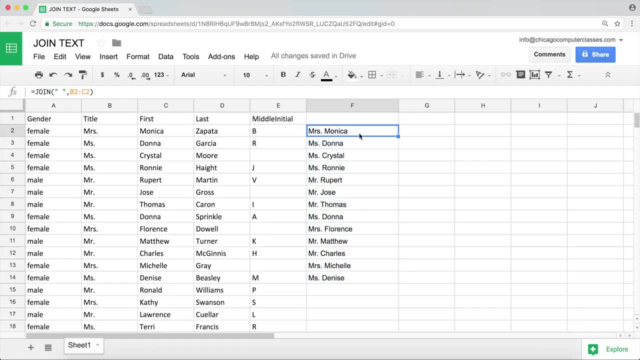 this is what I have now. the next thing I want to do, I want to basically join this with a period after that when this exists, and otherwise just not use that period, right? so I'm going to leave this alone for a second. I'm going to go here, I'm going to start with my equal sign and I'm going 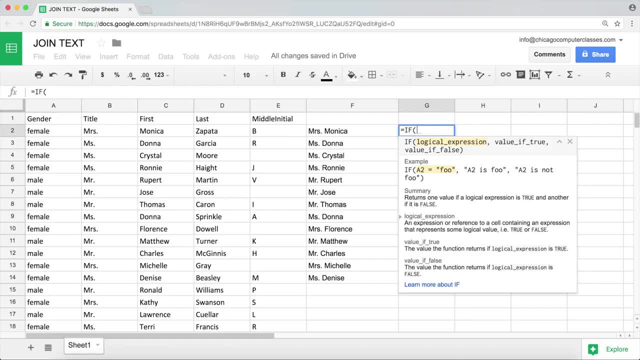 to start with a function called f. I have a video about if and ifs functions that covers a lot of details about this, but for right now, what I'm going to say is I'm going to check if this cell is blank, right, if there is anything in it. so there's a couple of ways to do that. so there's a function called is. 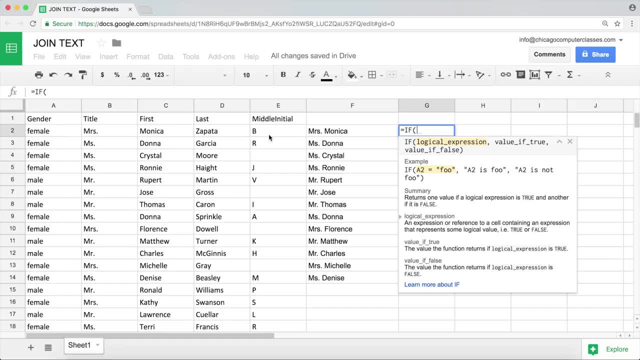 blank, that checks if a cell is blank and returns true or false. or there's also a way that you can say: if this is basically equal to nothing, and that means basically, if it's empty, right then what do we want to do if it's empty? basically, if that's the case, then we're going to say: if this is, 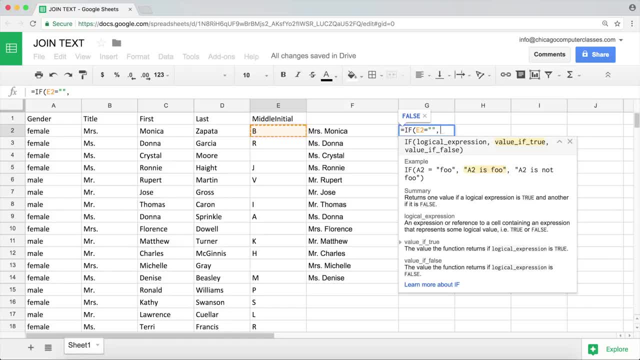 empty. we don't want to do anything, we just want to leave it alone. right, that's what we want to do. well, technically, we still want a space, probably in there, so I'm still going to do a space if the cell is empty. if the cell is not empty, however, I want space. I want a period, then a space, because I want 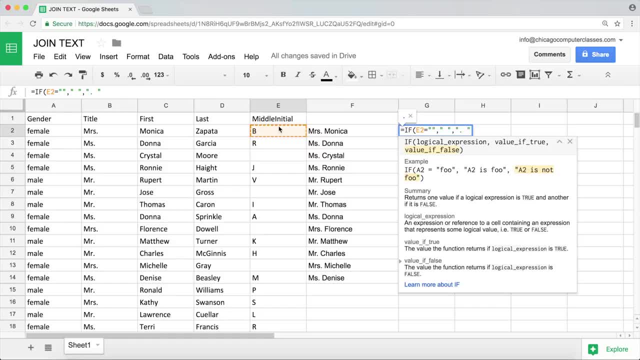 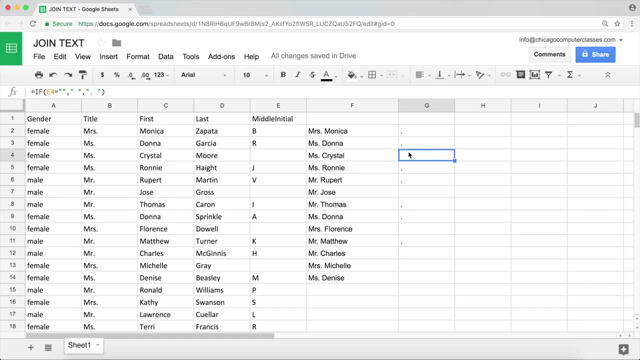 a period after that middle, initial, or I just want the space. so if I just enter so you'll see how we get a period or we should get. well, we get a space here and we there is a period after that. so just to show you what happens here. 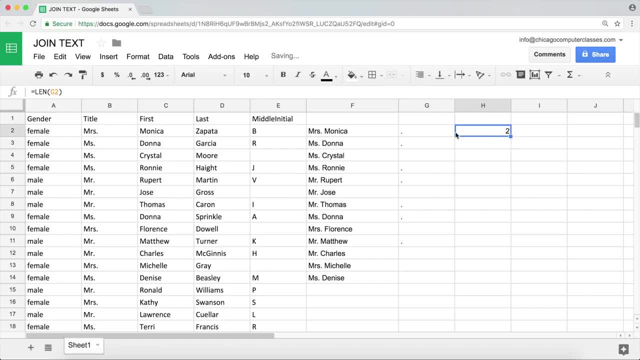 if I just check the length of this, see, it's the two characters, because it's a period and a space, and this is a one character because it's just a space. so that's what our if function is doing: it's adding the period and the space after that. 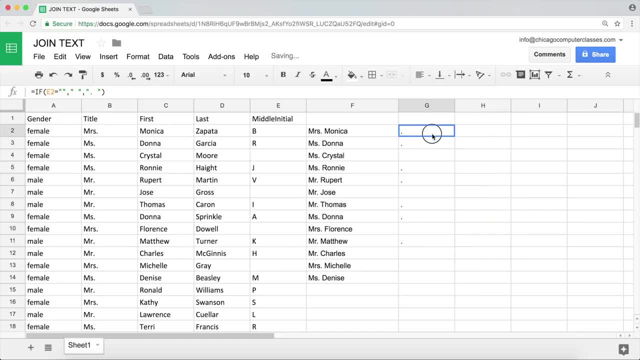 so clean this out. so now what I'm going to do. I have this if function. I'm going to copy that without the equal sign, escape out of it and go back here and I'm going to use my and sign, which is the plus sign, right and. 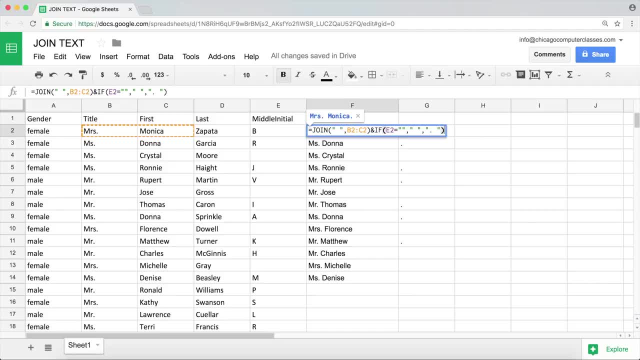 join that function right after that. so again, that and sign is like a plus for text, right? so we're joining that to this. so one thing I forgot to do is the actual middle initial, apparently. so i'm going to go back here. so what i wanted, i want. 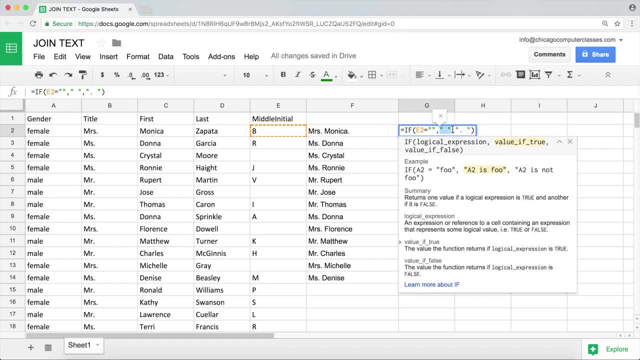 a space if middle initial doesn't exist. but when it does exist, i want it to be that middle initial, followed by that period and a space. right, so the middle initial is going to be need to sell and then again we do the plus sign for text and we join this. so i'm going to hit enter. 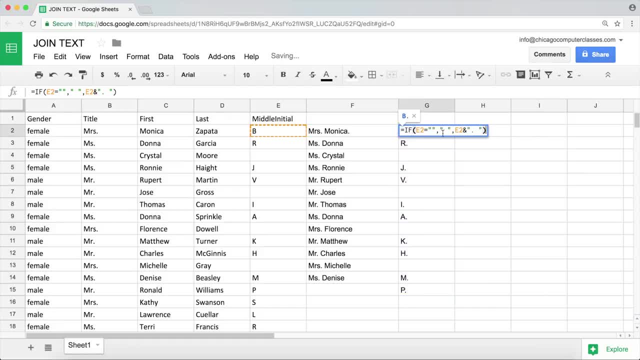 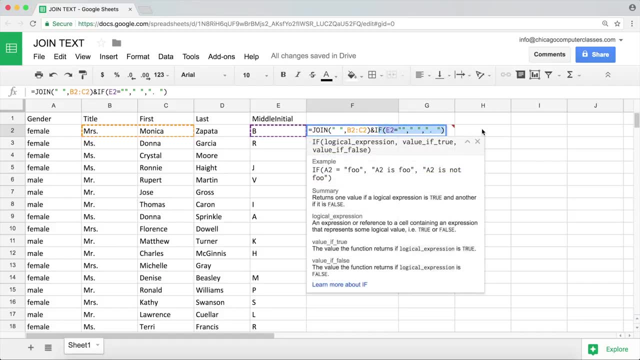 so copy this down just to see what we get. so that should work. so copy this, hit escape, go back and i'm going to replace this if function, which was almost right, but not completely right over here. what i did? i did a space, but it turns out i also needed another space before my initial. 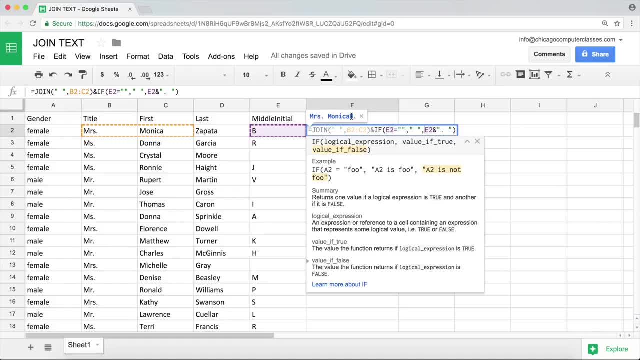 right here we can already see the results. so i need the title and the first name, then i need a space, then middle initial. so to add that space, i'm going to go: this is our middle initial, e2, and i'm going to do another space and another plus sign that should join a space. 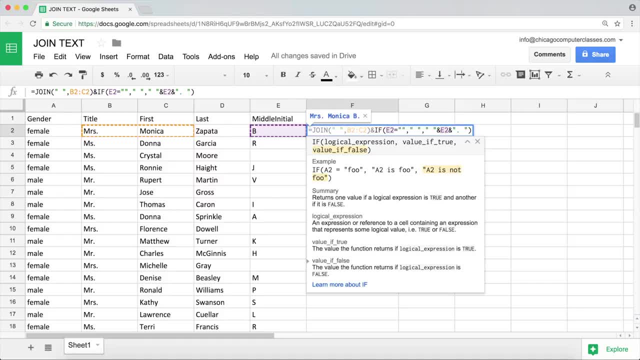 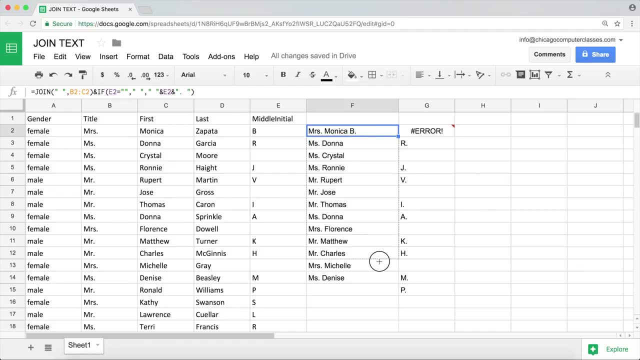 then our middle initial and then a period and a space if there is a middle initial. otherwise we could just add a space in there. so i'm going to hit enter, copy this down now. i shouldn't need this, so i'm going to delete that. so that's so far. 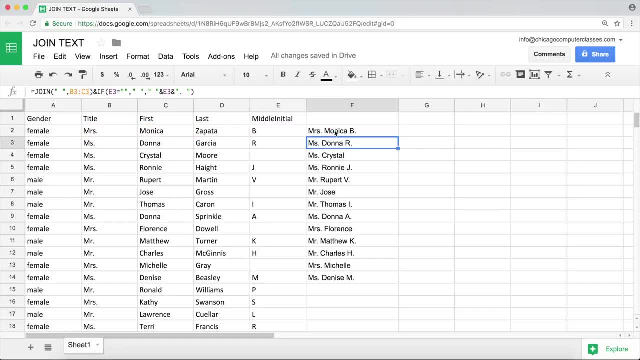 the title and first name, middle initial with a period or simply just a space if there isn't one, and then all i have to do in the end i have to also join the last name. so i'll do another and sign which is another plus right, and i'll join the last name. after that i'm gonna hit enter- go here. 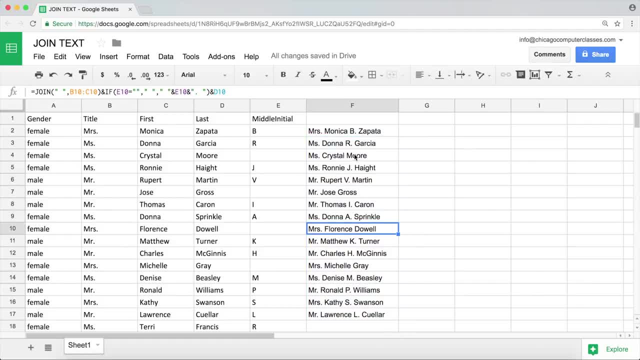 move this down, and now we should have what we need now. that's one method to do this now, another way i could have achieved this is by doing something like this. so the first thing i'm going to do, i'm simply going to use again my join function and i'm going to add my delimiter, which is a space. 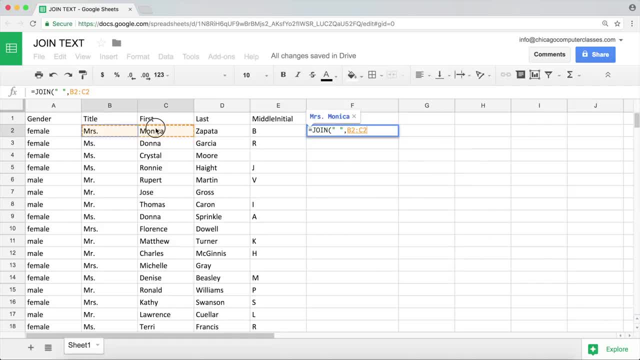 and i'm going to add title and the first name, and And after this, what we want is that middle initial. After that middle initial, I'm going to add a period and a space. After that, again, I'm going to add the last name. 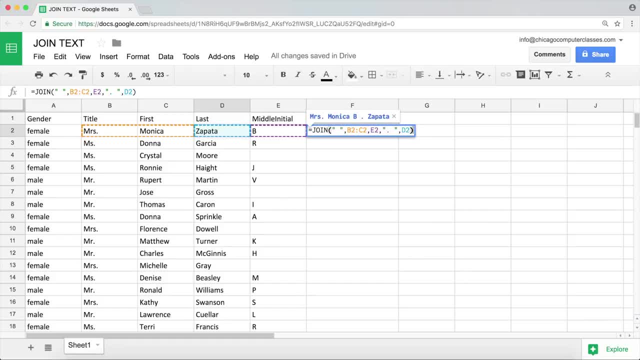 So so far, that's what I'm doing. I'm just basically using join And as one of the parameters in join I'm just using my own text, right? I'm saying let's do this, then do this, then do this period thingy we have. 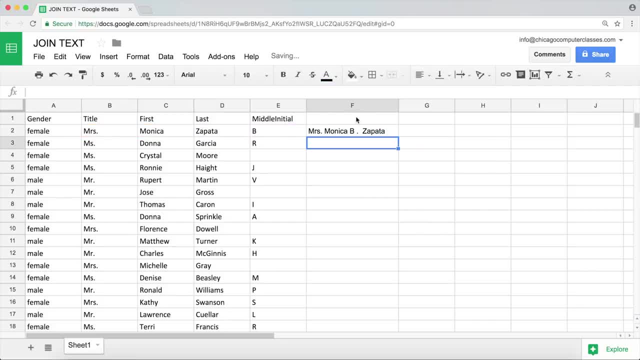 and then do this: Go ahead and hit enter. So that should give us this. Now you can see how I get this extra space between B and the period. The reason I get that, because I included this as a separate argument here, right? 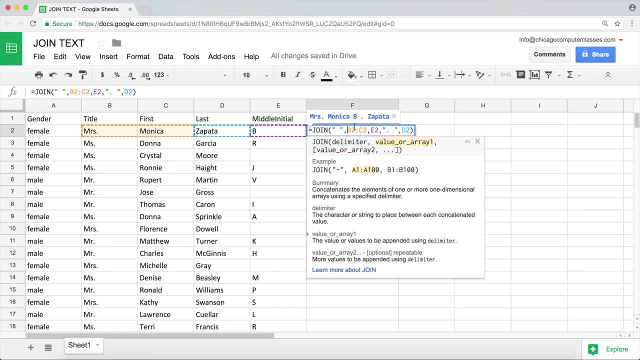 So, basically, and what it does? it basically takes each one of these pieces and it adds them together using this delimiter, which is a space, And that's why we should get actually that extra space. Now I should be able to just take this: 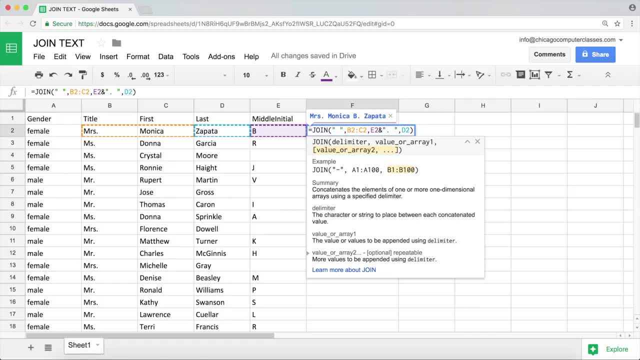 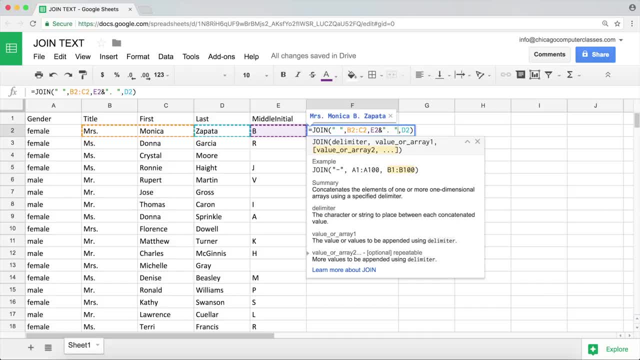 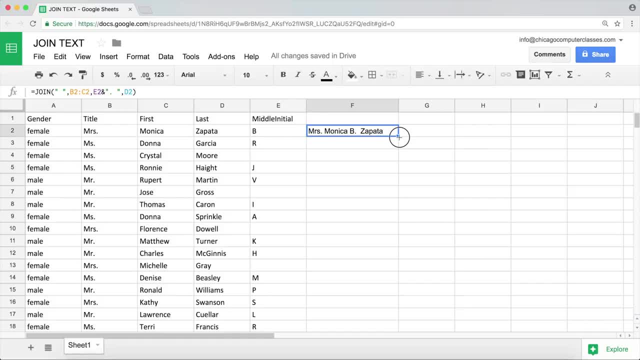 So I'm gonna hit enter So that should give me that title first initial, then our basically middle initial with a period, then a space and then a last name, right? So that's what we have. I probably have two spaces there. 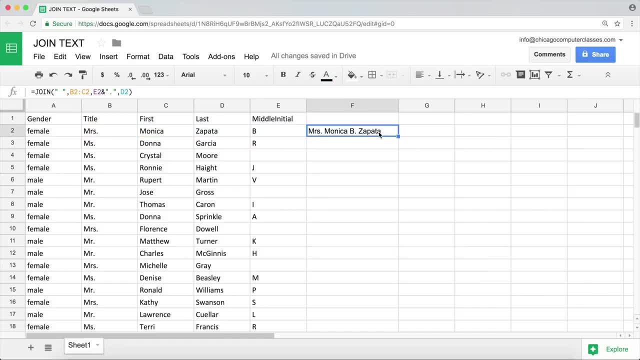 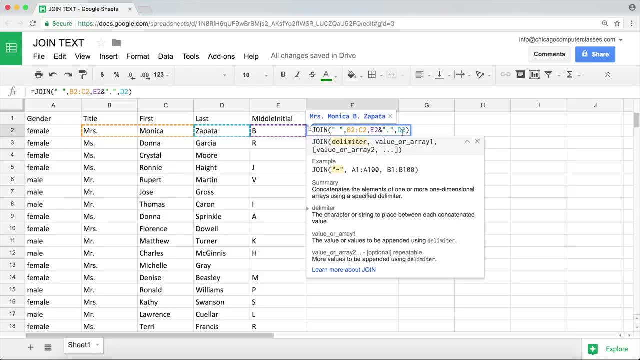 I don't need this space, So I don't know why I did that. but we just need the period, and then the space is gonna be created by this delimiter As another argument here. So that's perfect. So this works for this particular case. 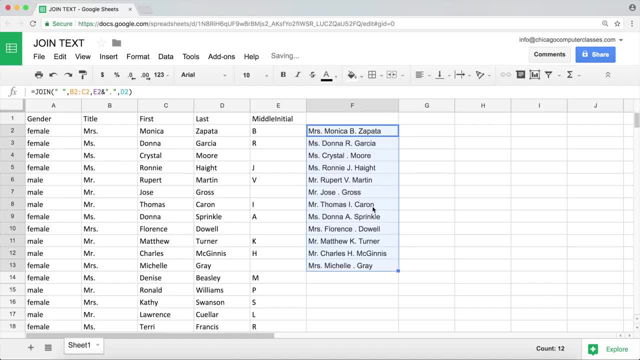 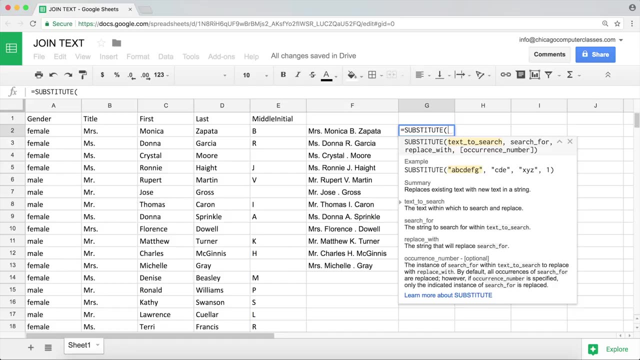 However, if I move this down, you'll see that in cases when middle initial doesn't exist, we get this period in the middle. So we have to handle that. So what I'm going to do, I'm going to use this function called substitute. 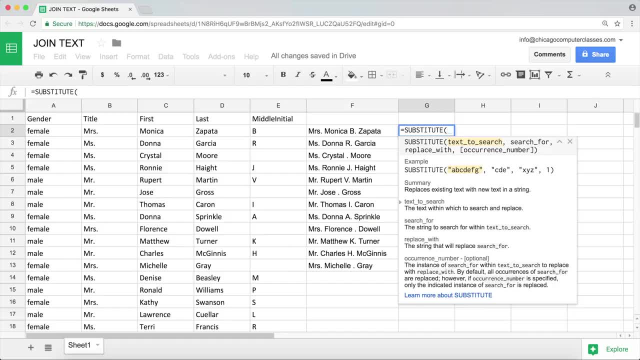 And I'm going to say, let's search for this text which is gonna be a space space period space. So over here there's no space period space, It's not gonna find anything, But over here we do have that. 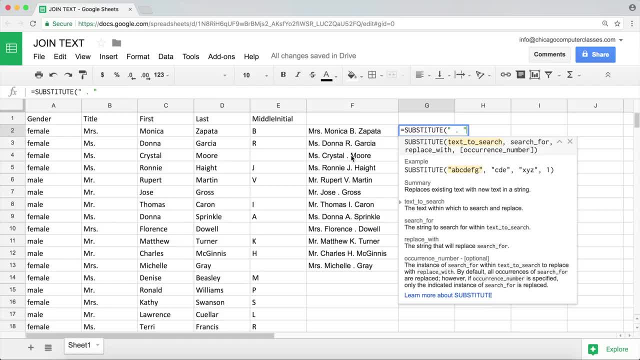 And I'm going to say: well, actually, the first argument here is text to search. So this is the text we're researching, comma. And the second argument is what we're searching for: space, period, space. And then I want to replace that. 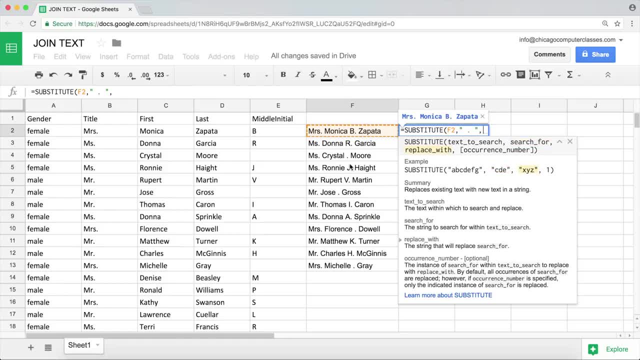 if I find it which is replace with, and then I want to replace that if I find it which is replace with. so, in this case, what do I need instead of this space? period space? Well, I need just a space. 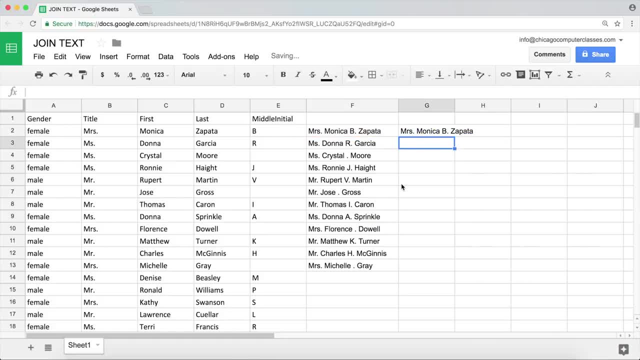 So I'm gonna replace it with just a space. So if I'd enter, well, it shouldn't do anything here, because it's not gonna find space, period space- But when it does find it- in this case, it replaces that with just a single space. 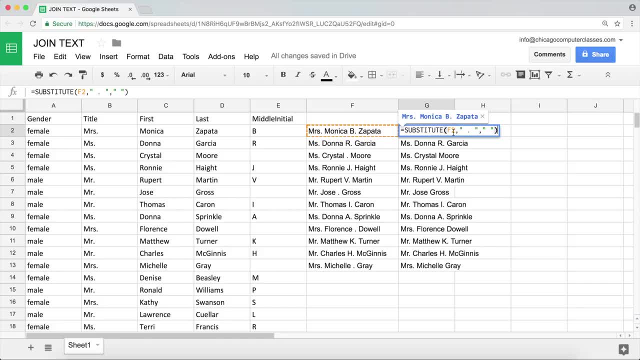 What I have to do. I just have to combine these two together. So right now I'm saying the F2.. So what is the F2?? F2 is all of these. So if I take this entire formula that I have, which is my join formula, 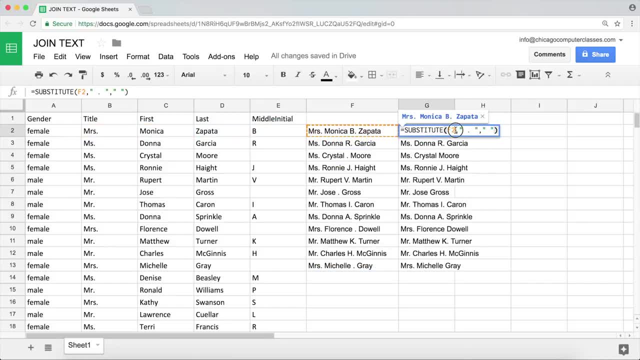 I'm gonna copy that: hit escape, go back here and I'm gonna replace my F2 with that complete formula: hit enter. I should get those results, but now I'm not connected to this, So I should be able to delete this column. 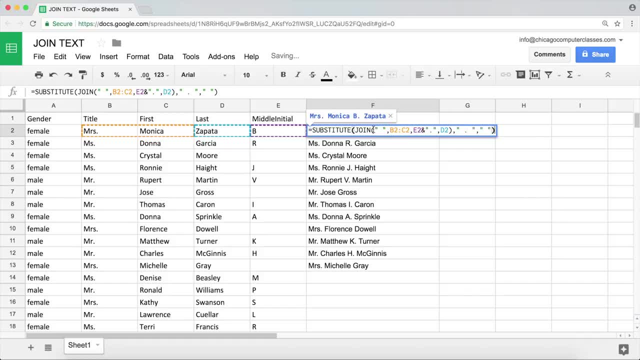 and still get my results. So that's another way which might be a little more cleaner, I guess. But there you are. So we have our titles: first initial, middle name, last name. So that's a couple of ways you can use to join. 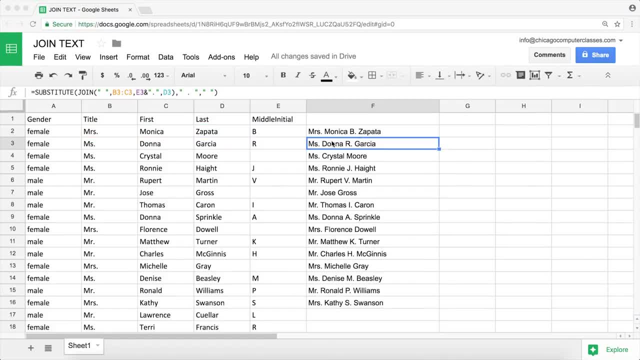 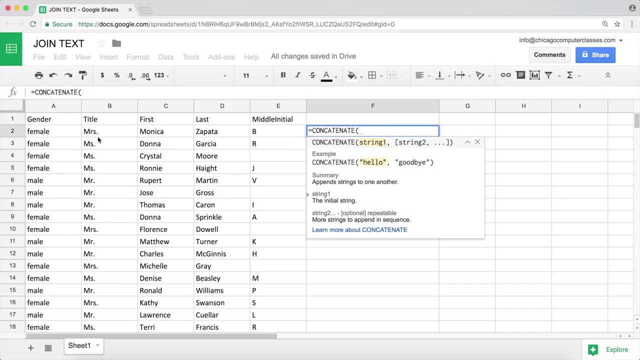 and do some string operations. So, finally, the last function I want to mention is the function called concatenate. You may see people using that, So I'm gonna use concatenate function. So the first thing is the title, So I'm gonna use comma. 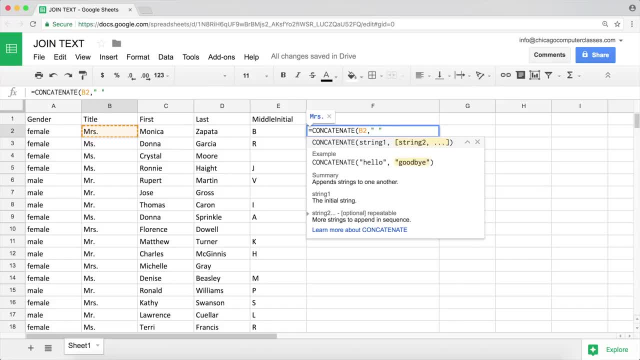 Then I want the space after the comma. So in this case there is no delimiter. like we provide one delimiter for every piece of text we have, You actually have to provide which is the next piece of text you want to join. So I'm going to do this title. 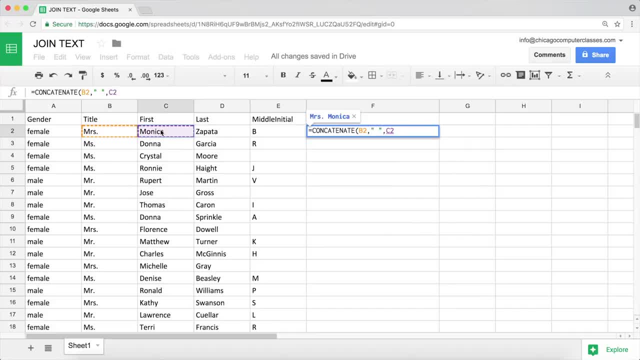 and then I'm gonna do the space, And then I want the first name. After the first name, I want a space, So another comma. then I want the middle initial, So coma again, the middle initial. we want a period space, comma again. and then finally we: 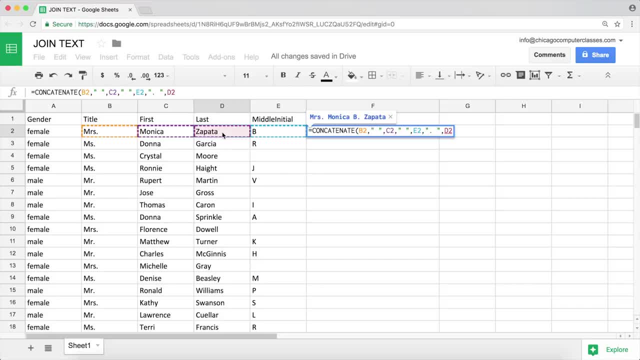 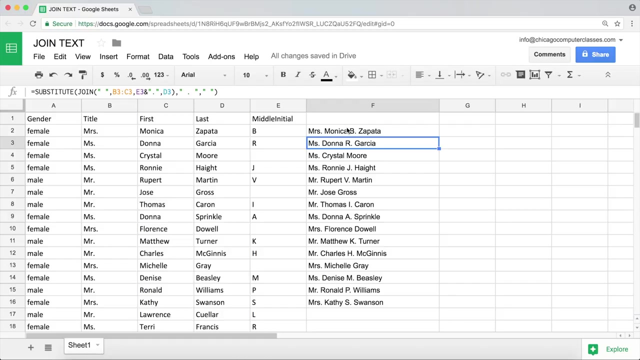 want the last name as the last piece. I'm gonna close that right here. so there we have it. that should do this and join them together. and again, I could fix this by using substitute function again to remove this space period space, but you already know how to do that. hopefully that was helpful. please subscribe and. I'll see you in my next video.